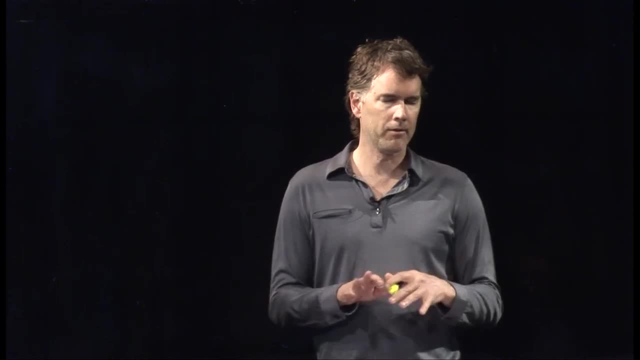 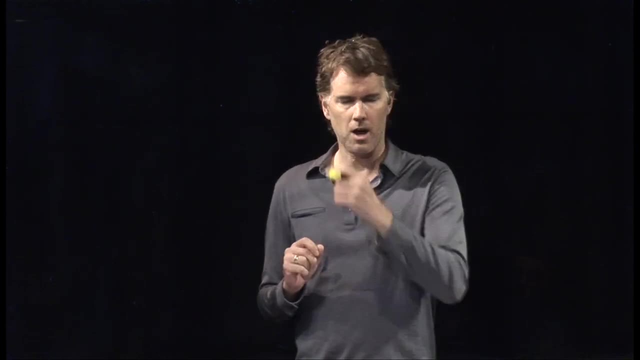 We, of course, live in a three-dimensional world, but a lot of the problems that you're going to face in physics are really two-dimensional problems. So, for instance, if you throw an object, that object actually follows two-dimensional motion. 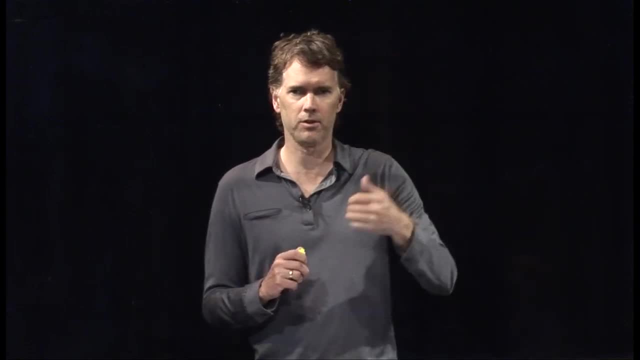 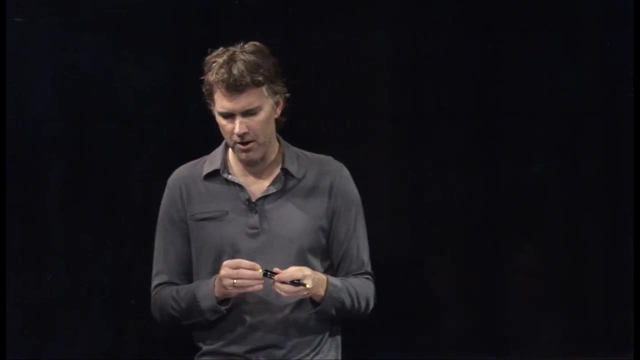 Okay, it has some x position, it has some y position, But it doesn't really come towards you or away from you. so there's no third dimension there. It's really a 2D problem. All right, so let's talk about two-dimensional kinematics. 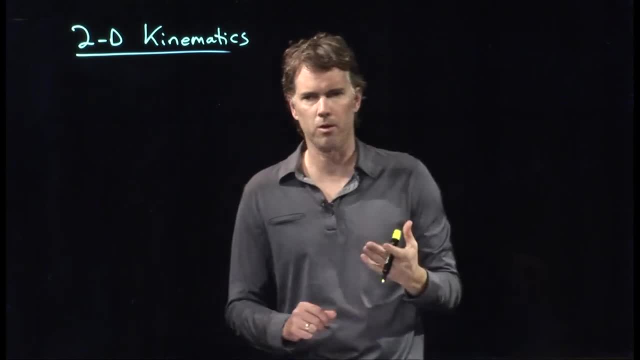 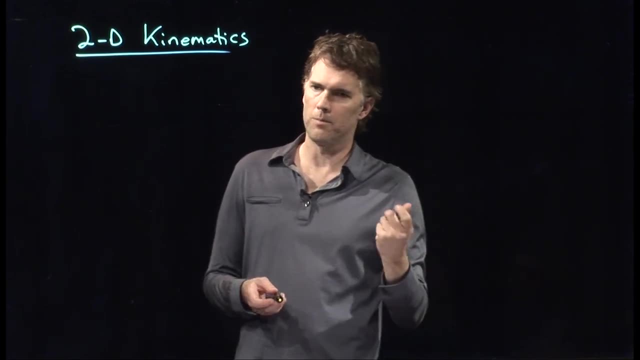 And let's approach this with the following thought experiment: Let's say that we go to the top of the Empire State Building and we take an object, say a marble, and we throw it off the top of the Empire State Building and we throw it off. 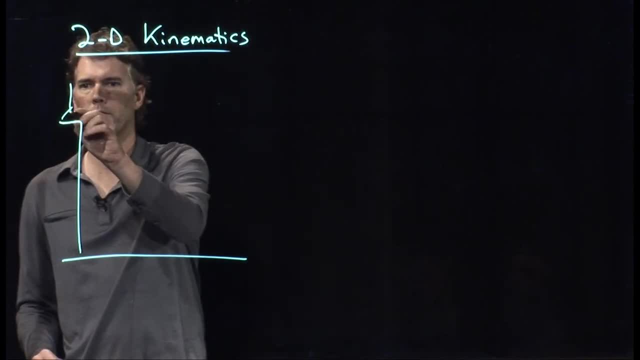 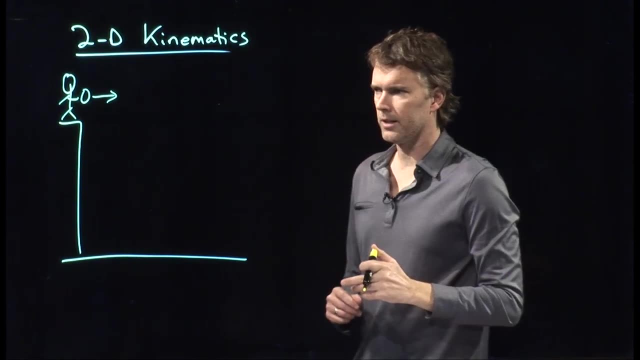 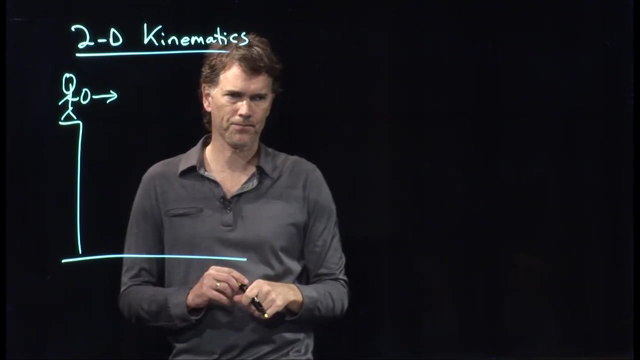 horizontally. You, of course, should never do this. I'm sure you'll get in big trouble if you do. But if I launch this object horizontally, what sort of trajectory does it take? Anybody know what that trajectory is called? Yeah, 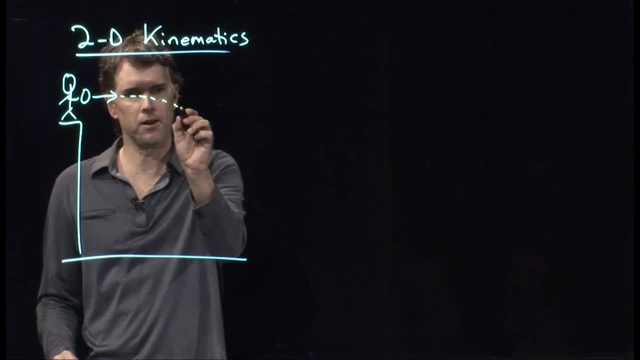 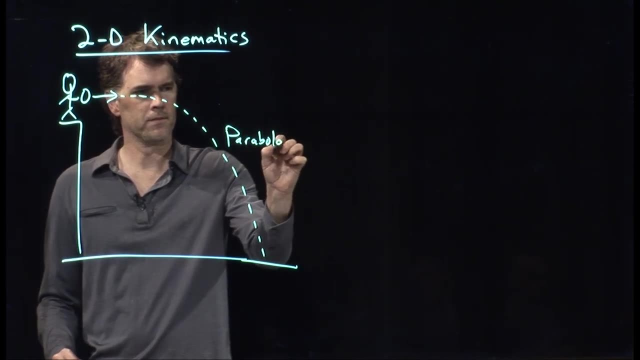 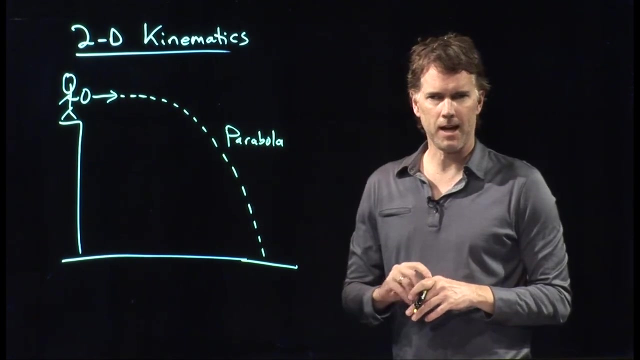 A parabola, right. It sort of curves down like so, and that is, of course, a parabola. Is there another name for this projectile after it leaves my hand? Is there another name for that type of motion? And I'll give you a hint. I just gave you the two words that are in the answer. 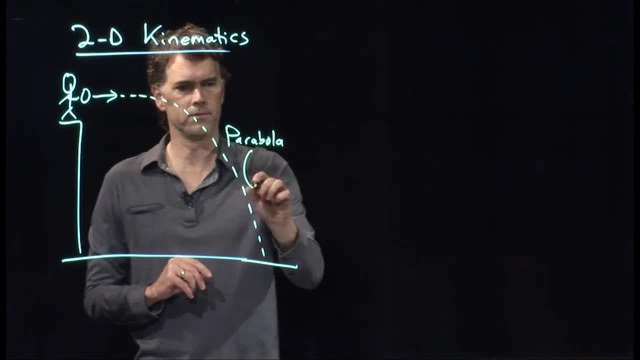 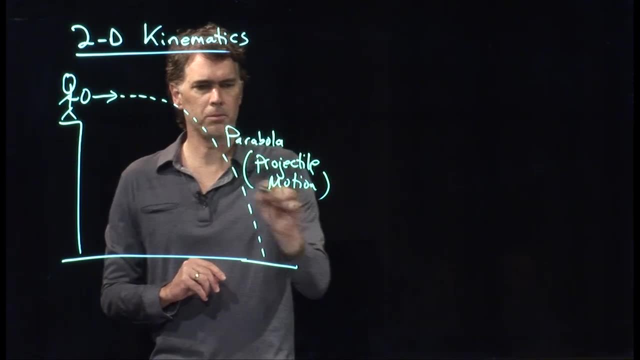 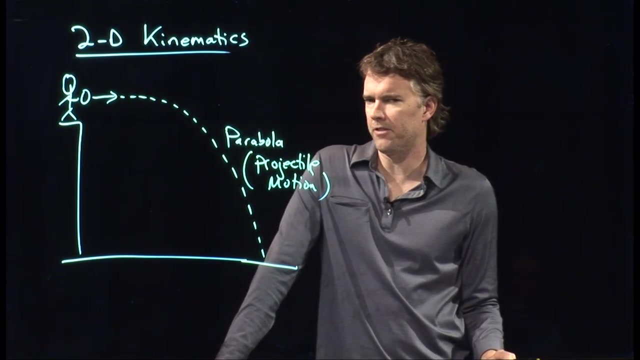 Yeah, Projectile motion. Okay, this is projectile motion. We have launched an object, it follows a parabola and it is projectile. That's what we call it. All right, so let's see if we can understand a little bit about this motion. 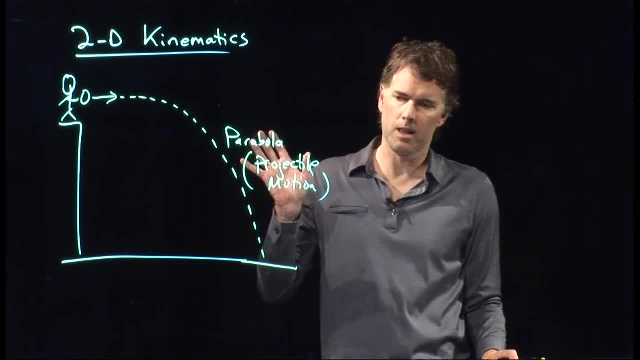 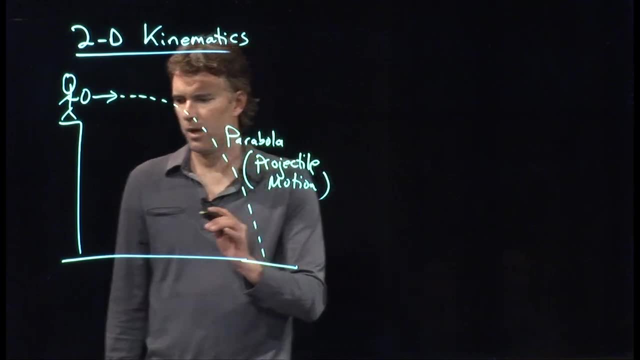 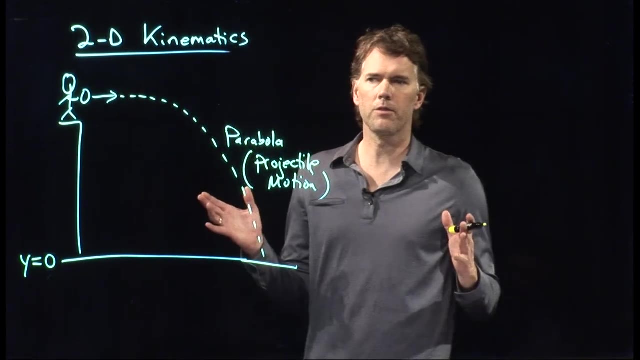 Okay, this is, of course, the motion that governs a lot of things as they move around near the surface of the Earth, And so it'd be nice to understand the problem. So, first off, let's draw a coordinate system. Let's say that y equals 0 is down here at the ground. You can, of course, make that wherever you want. 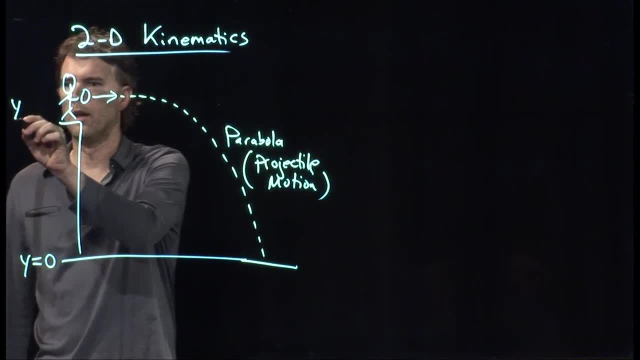 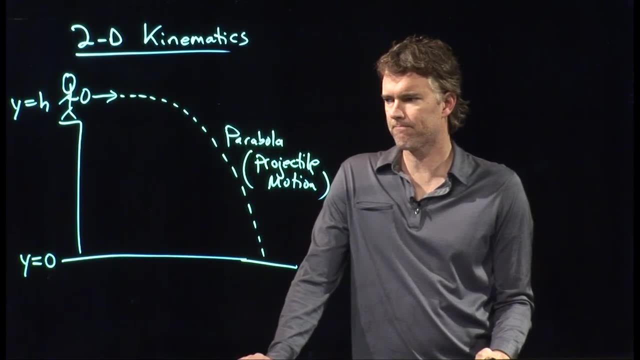 but that seems like a natural starting point Where we launch the object from. let's say that is: y equals h. All right, Now what do we do? Well, let's think about this motion for a second. First off, why is it curving down? 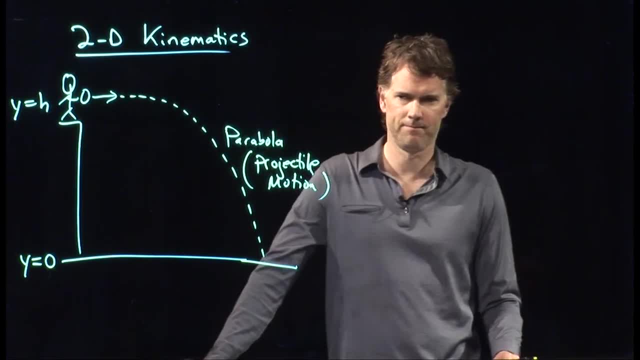 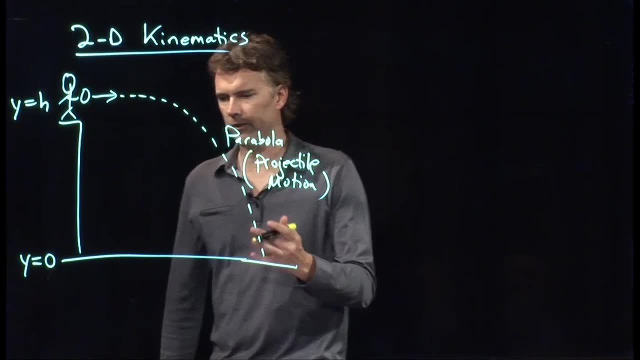 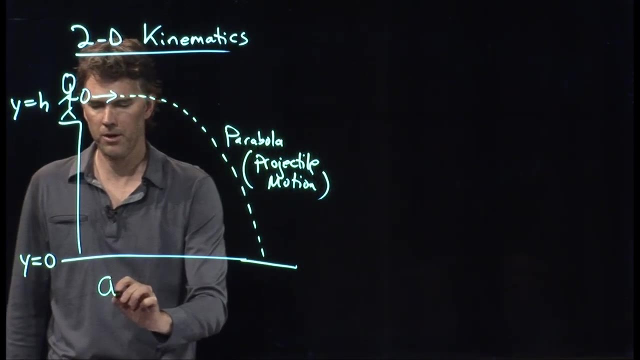 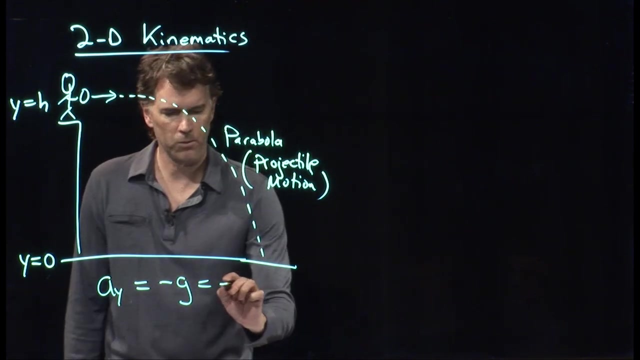 What is dragging this thing down towards the Earth? Yeah, Gravity, Gravity. Gravity is, of course, pulling it down towards the Earth. No, gravity thing just keeps going on forever and ever, and so gravity is really important here, and, in fact, the acceleration due to gravity- we know it is negative g, which 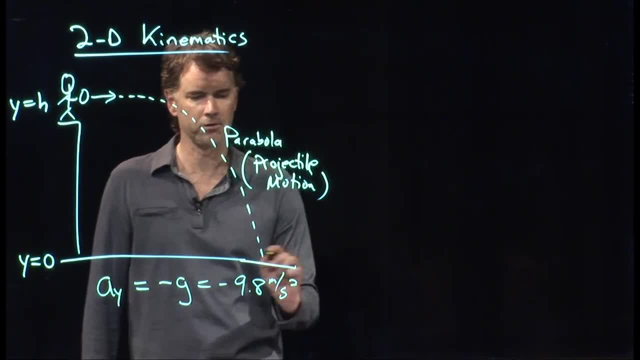 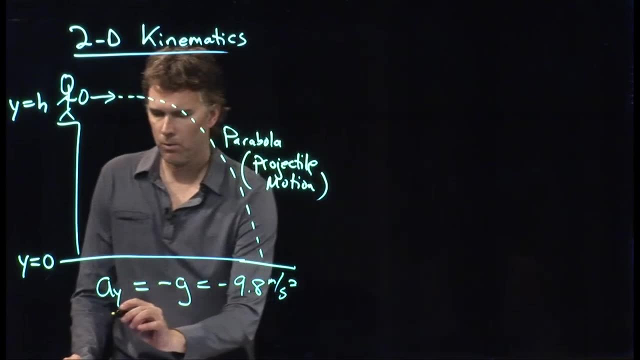 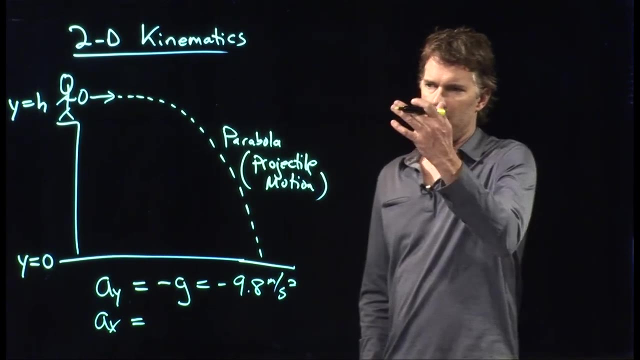 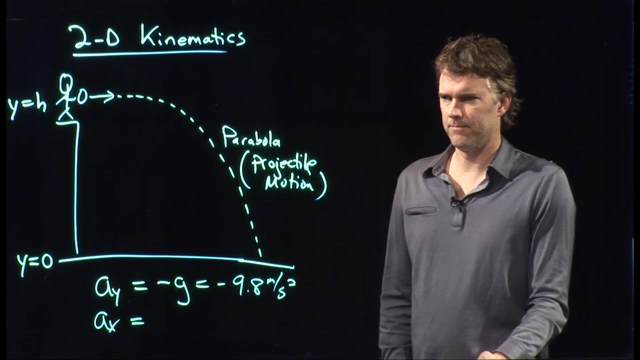 is negative 9.8 meters per second squared. What about the other dimension? What about the x dimension? What is the acceleration in that direction? Does anybody know? Yeah, over here on the left, Zero, Zero. Why is it zero? Because x is going flat. 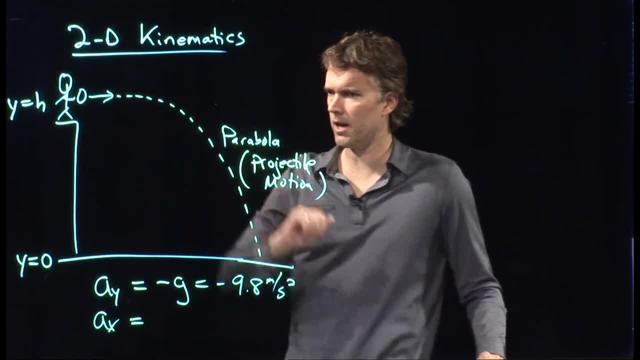 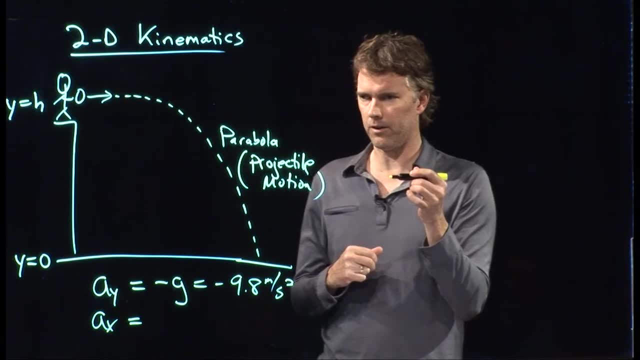 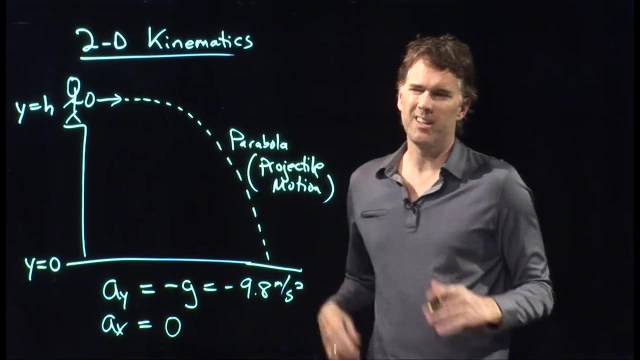 Because x is horizontal. Yeah, Okay, and, as we're going to learn later, there is no force in the x direction. Okay, the only force here is gravity, which is downwards, and so, in fact, there is no acceleration at all in the x direction. if we're 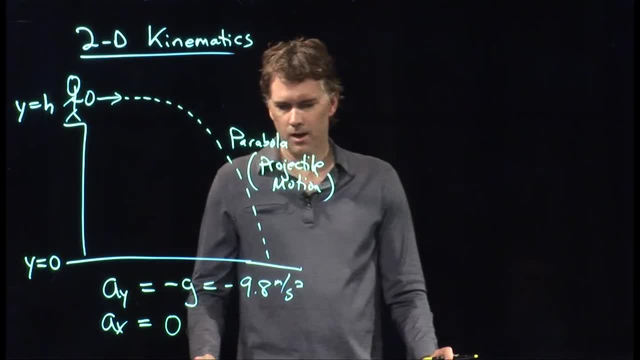 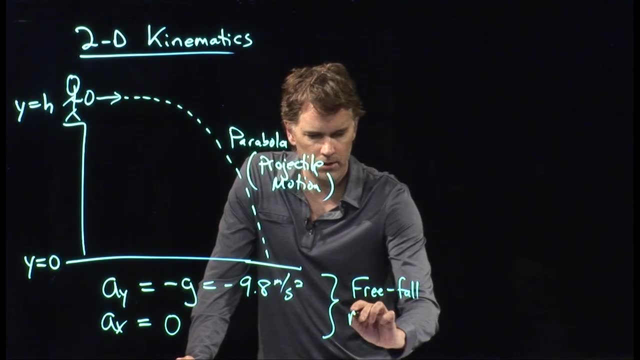 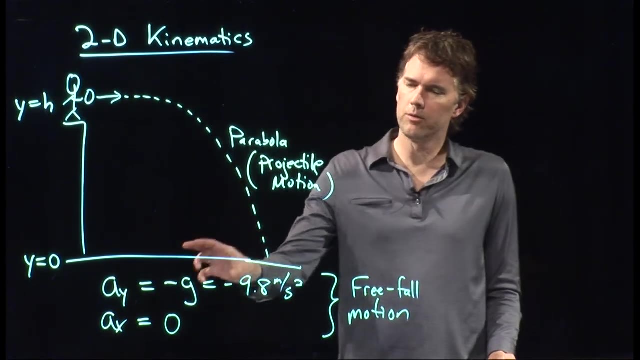 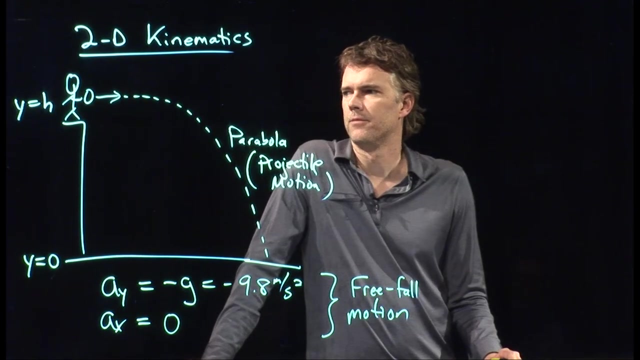 ignoring that. We're ignoring air resistance. okay, which we are. Okay. this set of conditions is projectile motion, or also known as free fall motion. When you are only under the influence of gravity, then you are in free fall. Okay, so now, what do we do? Well, let's ask the question: how? 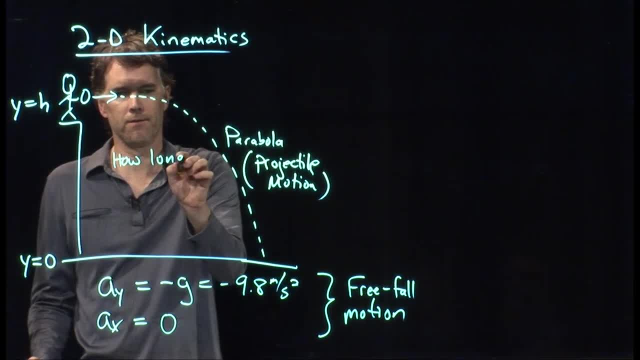 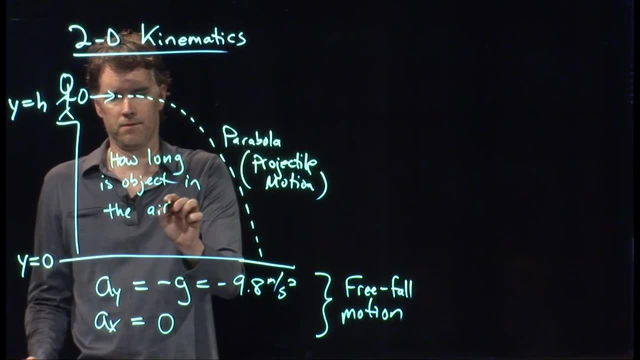 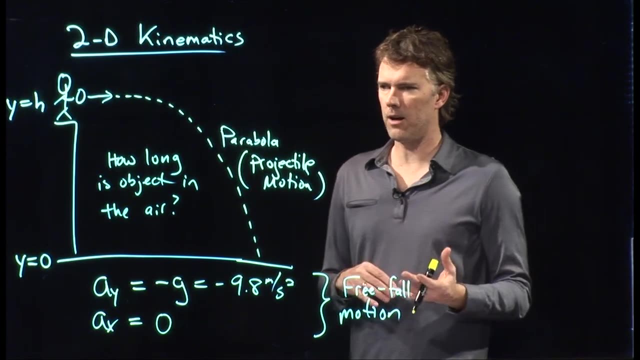 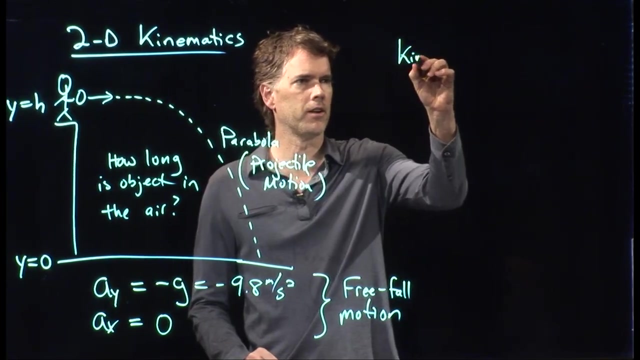 long is this thing in the air? How long is that thing in the air? How do we deal with this problem? Well, we've learned a lot about motion in one dimension. We've learned about the kinematic equations. Let's just go back to the kinematic equations for a second and see. 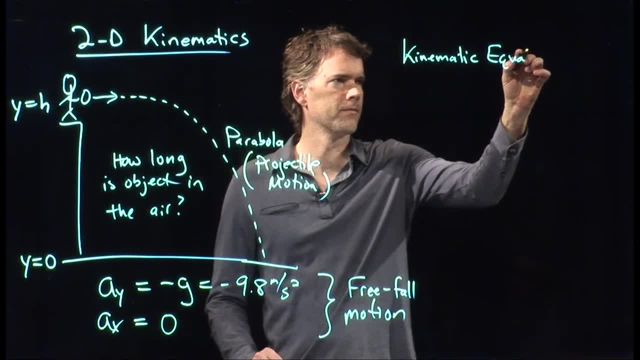 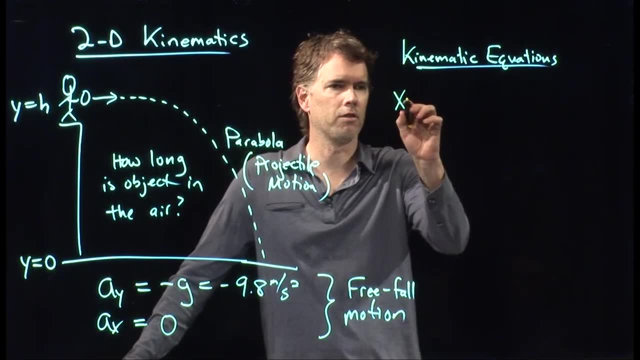 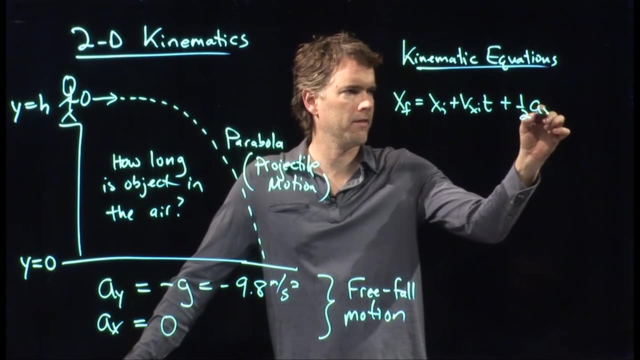 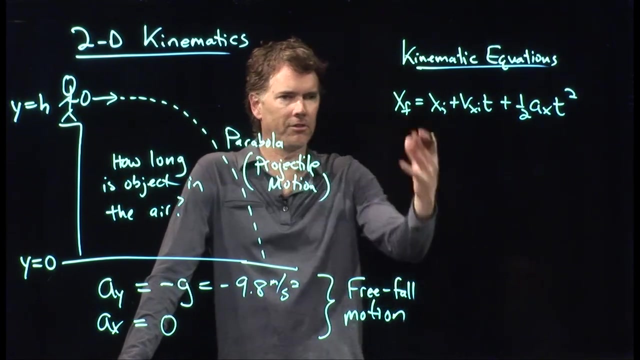 what we have? Okay, All right. what we have is equations like this: X final equals x initial plus v, x initial times t plus one half a sub x, t squared. All right, that looks pretty good, but x is just some variable. All right, it could be whatever variable I want, so let's just change it to something. 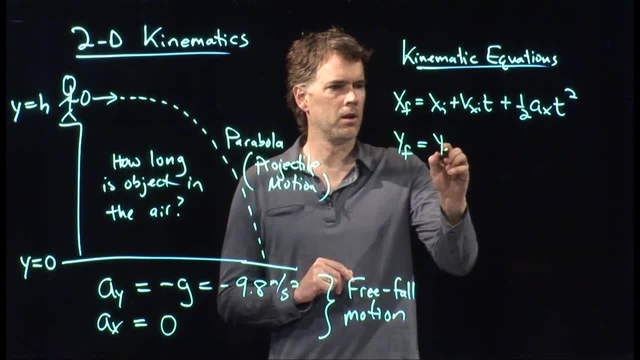 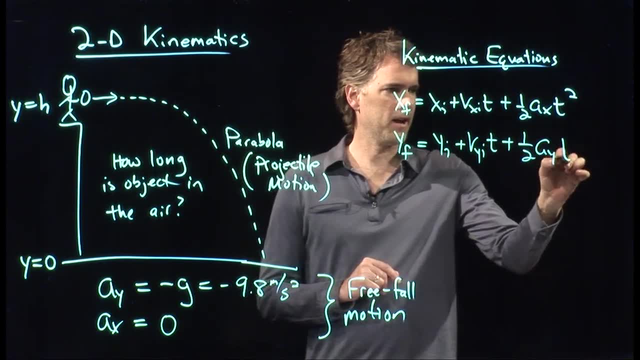 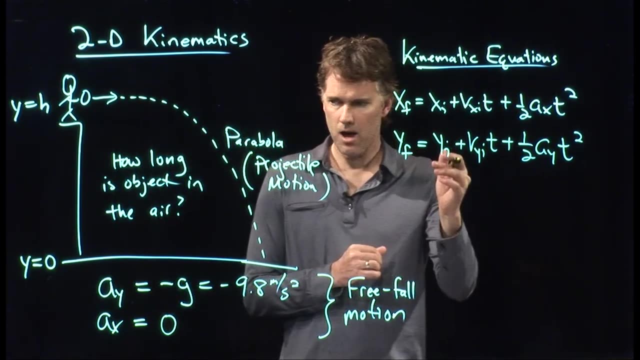 else Let's change all of those x's to y's, Y final. All right, Okay. So y initial equals y initial plus v y initial times t plus one half a sub y, t squared. That seems perfectly valid. Okay, And now? I like this because we usually say the vertical. 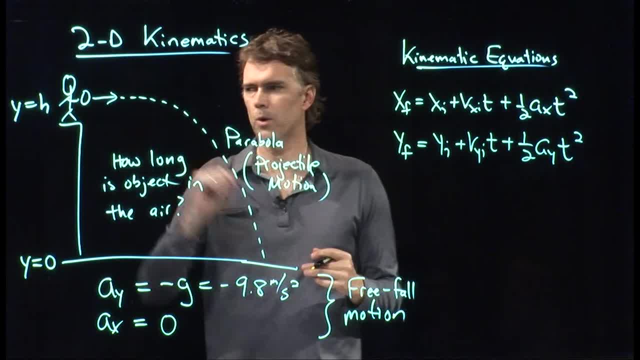 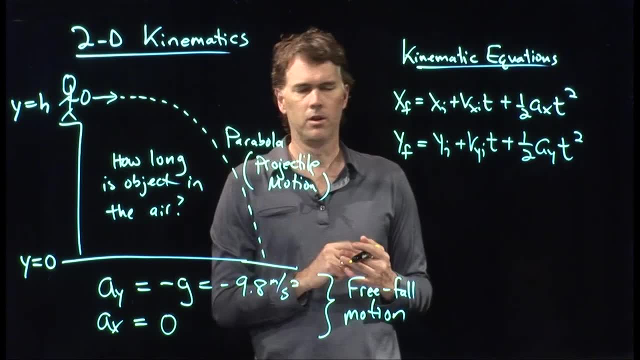 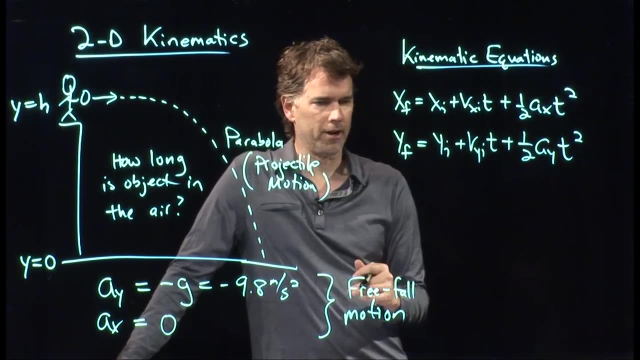 position is y, and in fact we said y equals zero is down there and y equals h is up there, and so this equation looks like it might be able to help us answer the question: how long is this thing in the air? All right, So let's take a look at this equation In our problem. what is y final? 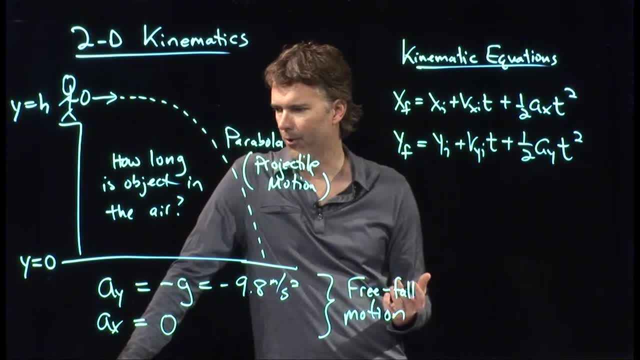 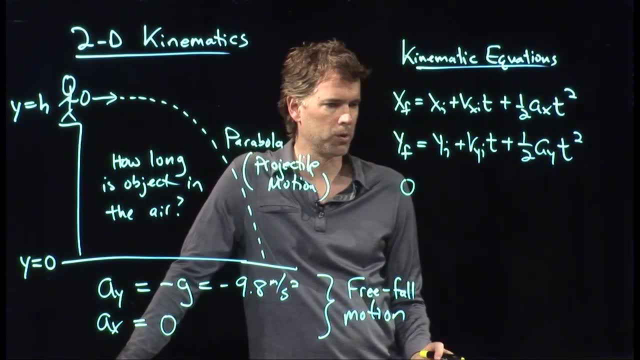 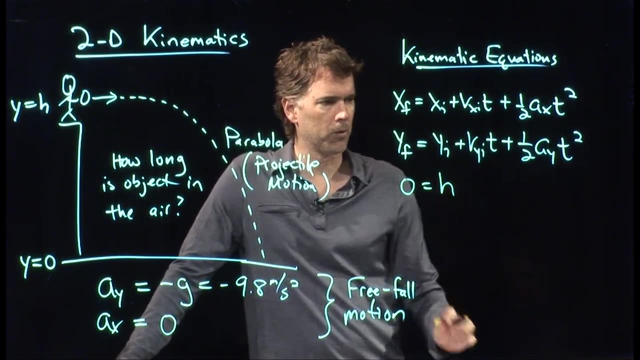 Yeah, what's y final? It's the ground, It's the ground, And we called the ground zero. All right, we could have called something else- zero, but the ground seems like a perfectly good choice for a height of zero. If the ground is zero, then where we started initially is, of course, h. What about? what about h? What? 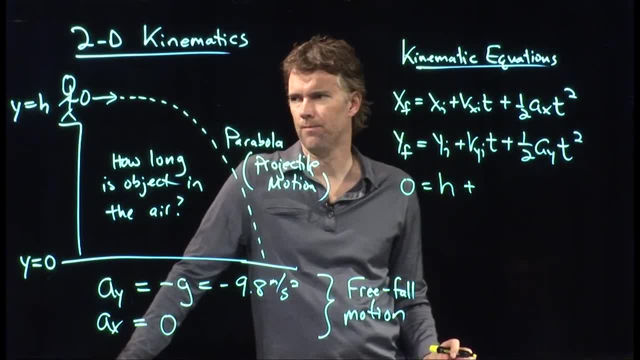 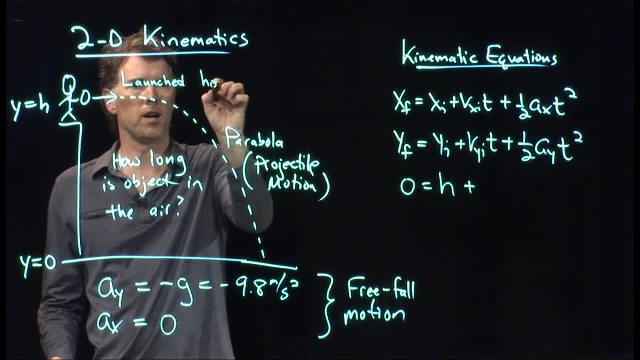 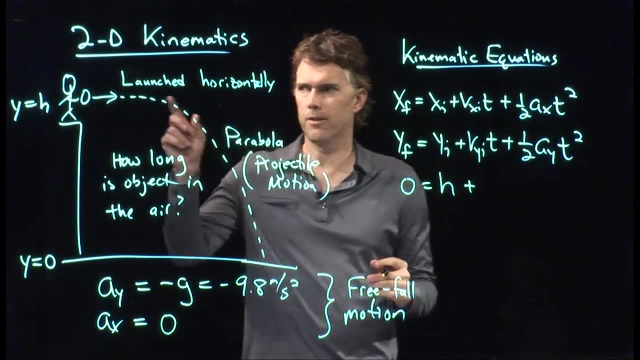 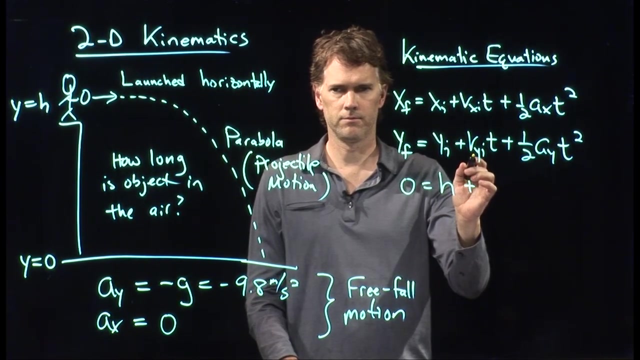 about the y initial And let's be clear here that we are going to launch this object horizontally. Okay, that's kind of key in our discussion at this point. If we have launched this thing horizontally, what is the vertical component of the velocity? Yeah, 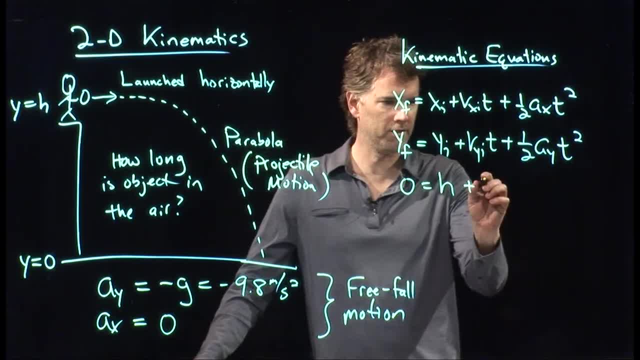 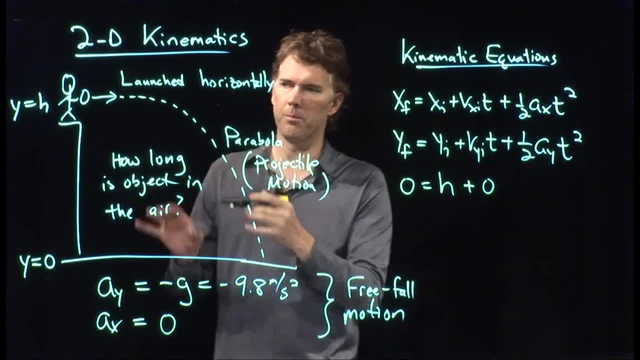 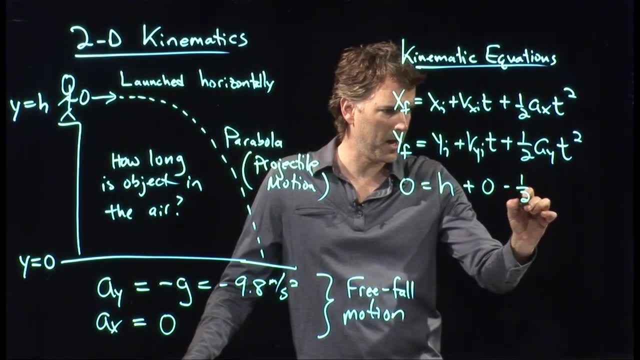 It'd be really hard to launch something perfectly horizontally. But let's say we do launch it perfectly horizontally, then that term is zero as well. And now we're just left with this One half a t squared. we said a was minus g, so I'm going to pull that out in front. 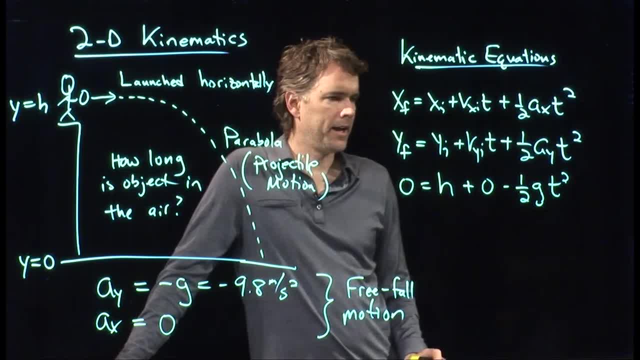 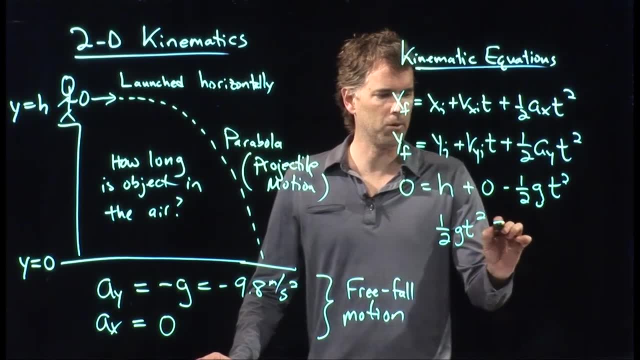 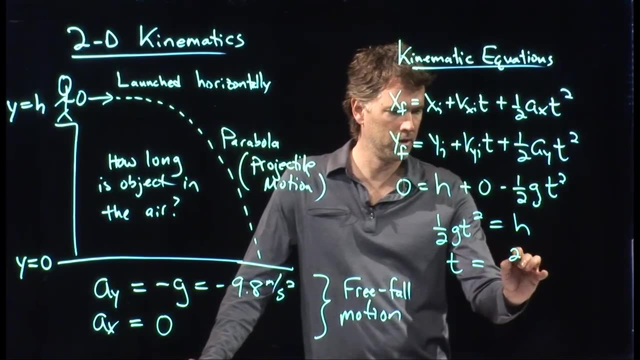 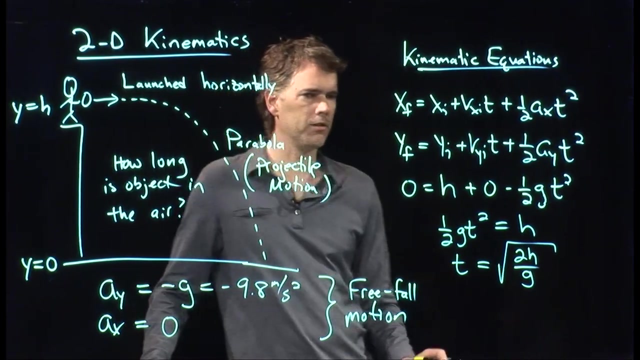 and I get minus one half g, t squared. And now, look, I can solve this equation for t. I'm going to move this over to the other side. I get one half gt squared equals h. and now I can solve for t squared: T, I multiply across by 2, I divide by g and I take the square root. This is the time. 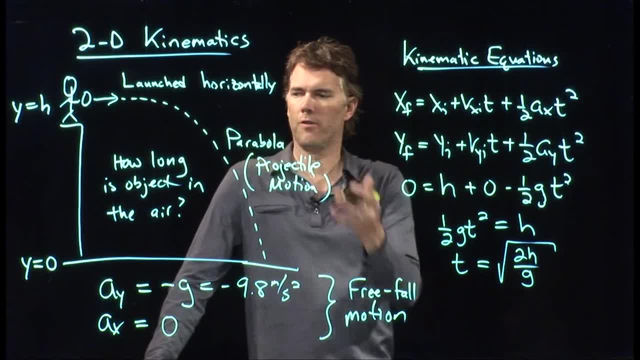 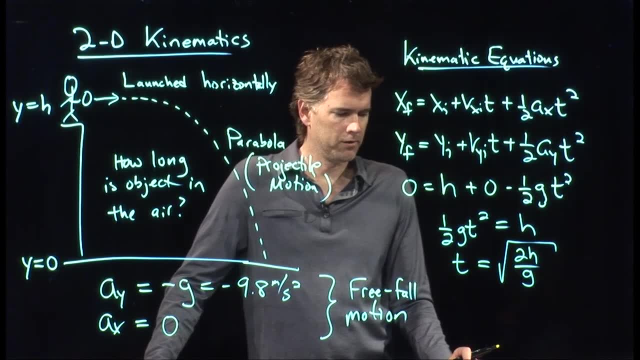 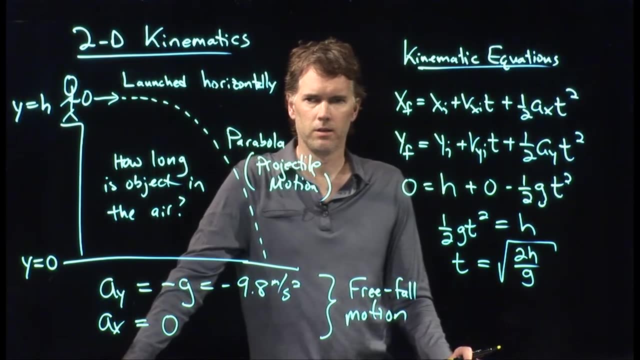 it takes for any object to fall from a height h, And there's something sort of interesting here, which is the following: Let's say we didn't just launch it horizontally, we just stood there and dropped it vertically. Would this time be exactly the same? Yes, because 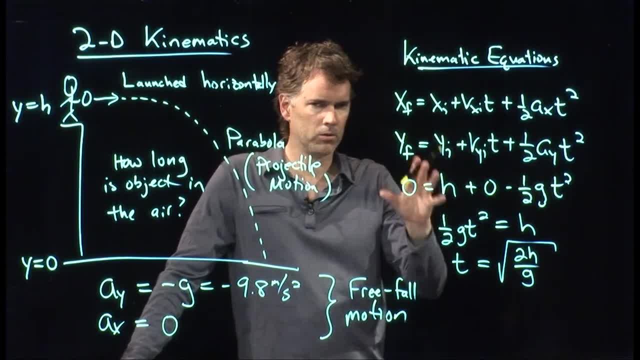 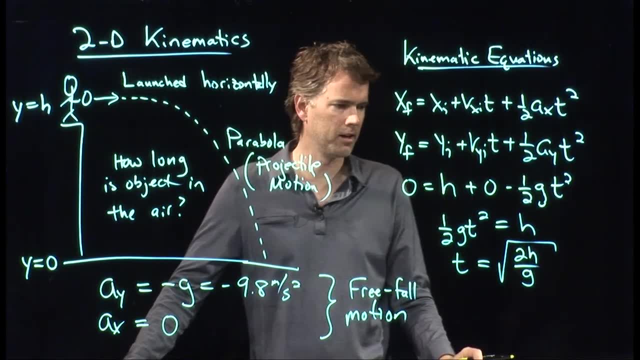 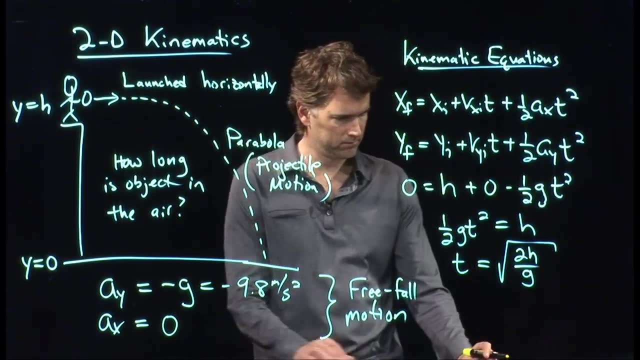 this equation right here is only dependent on the height that you started from. Since we have zero vertical component of the initial velocity, we would get the exact same time, And now we can plug in some numbers and try it out. Okay, so how high is the Empire State? 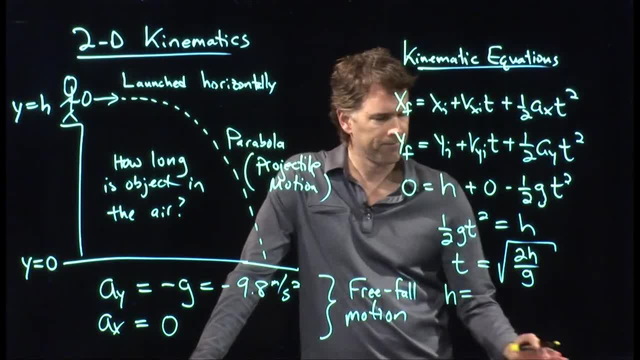 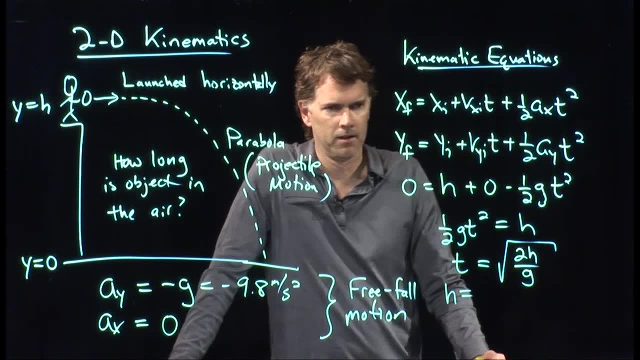 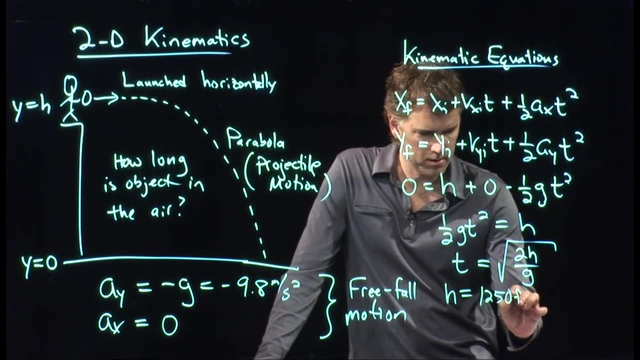 Building. Somebody told me this earlier. They looked it up on their phone. How high was the Empire State Building? It's about 1,250 feet. 1,250 feet, Okay, And that is, of course, English units. We like SI units, So let's. 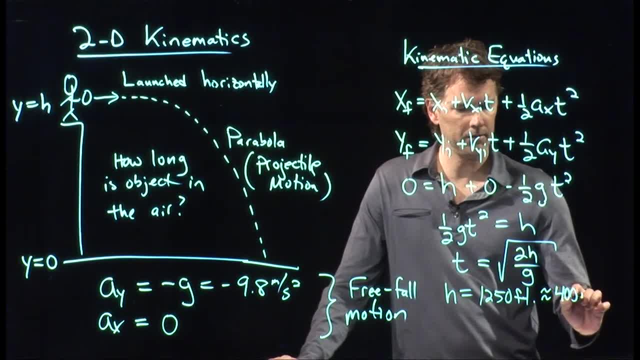 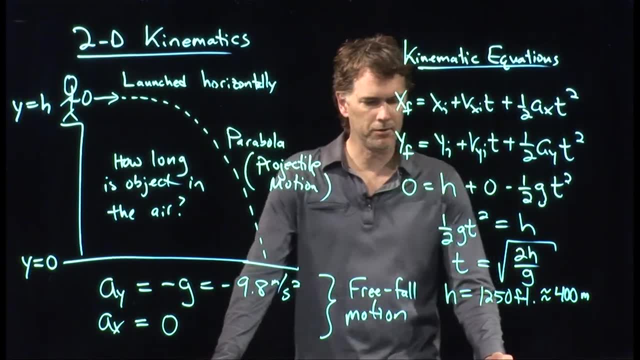 just approximate that as 400 meters. You can do your calculation yourself and see if that's pretty close, but I think that's pretty reasonable. Okay, And now let's see if we can calculate the time t we said was square root of 2h over. 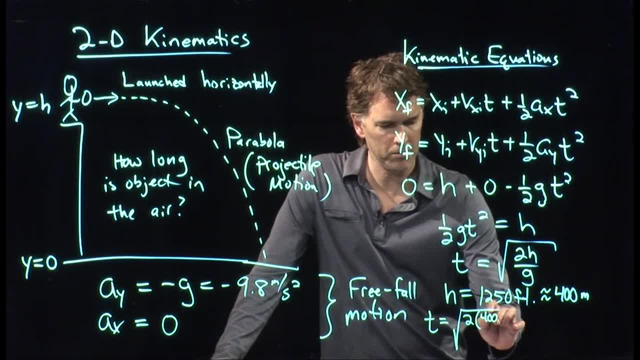 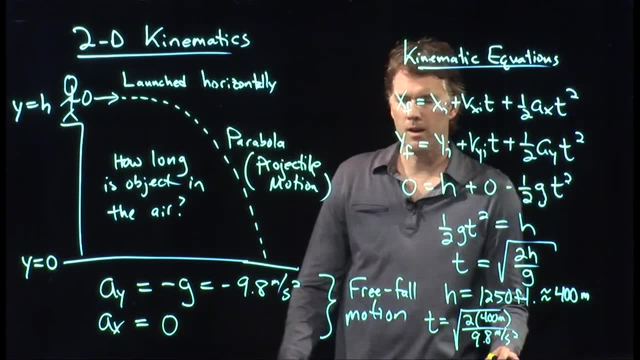 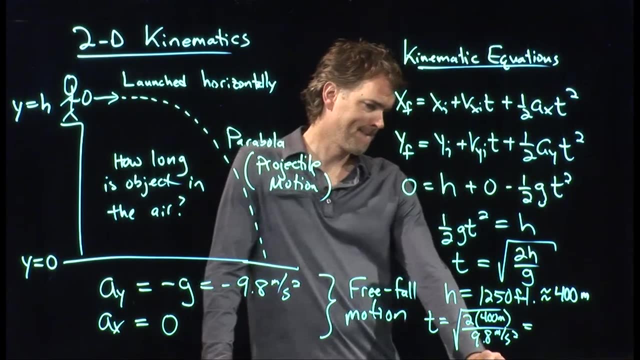 g. So it's 2 times 400 meters divided by g, 9.8 meters per second squared. And now we can run this in our calculator or we can just approximate it: 2 times 400 is 800.. 800. 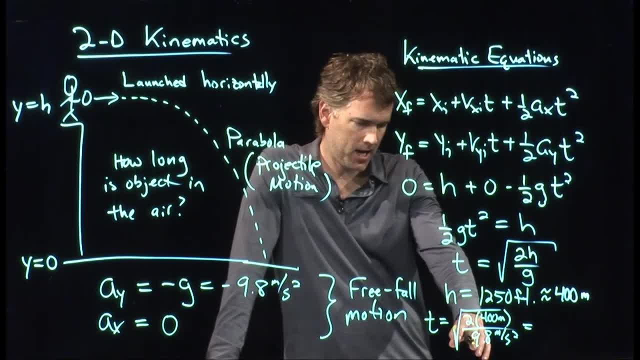 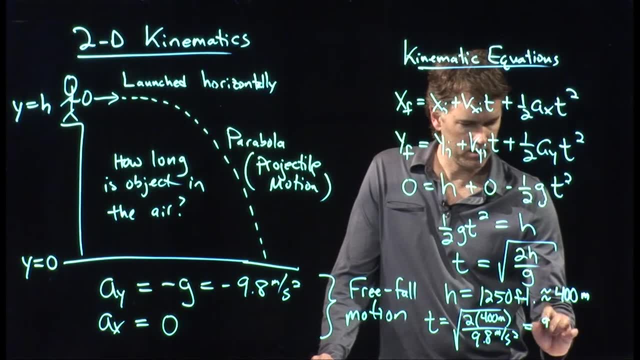 over 9.8 is pretty close to 800 over 10,, which would be 80. Square root of 80 is about 9.. So I would say 9.. And did anybody run it on their calculator and get an exact answer? 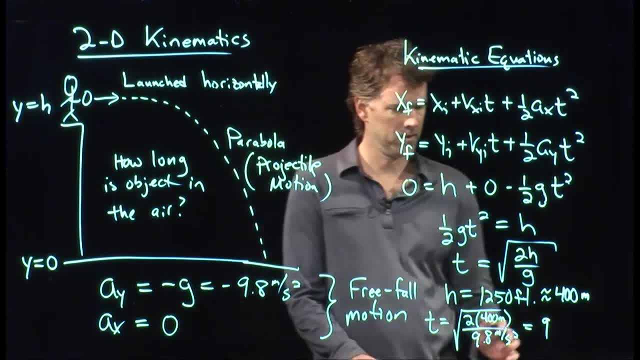 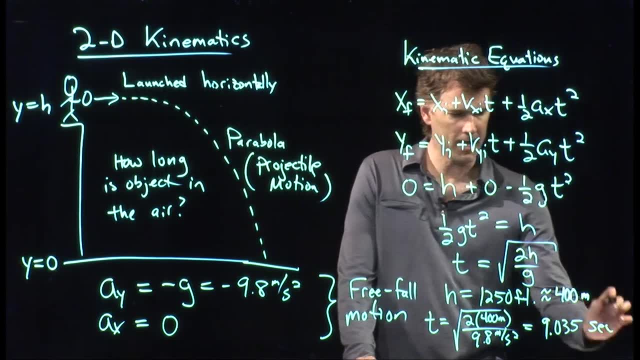 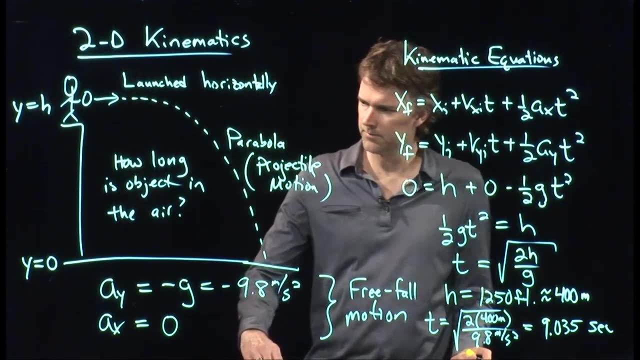 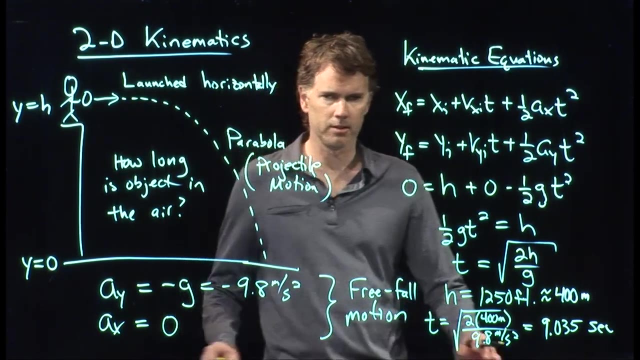 Yeah, what did you get? 9.035.. 9.035 seconds, Okay, So pretty good. guess we had for 9 seconds, And that's how long that thing would be in the air. 9.035. Okay, 9 seconds, All right. Hopefully that one is reasonably clear. If not, definitely.